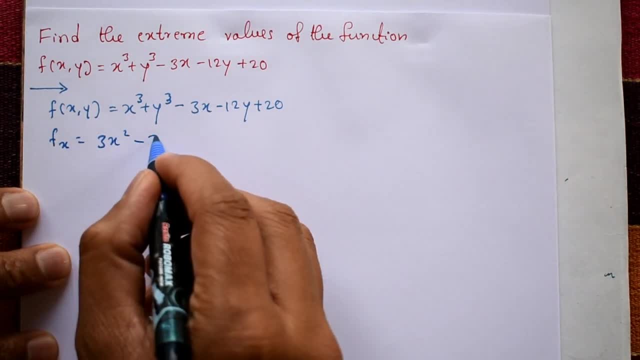 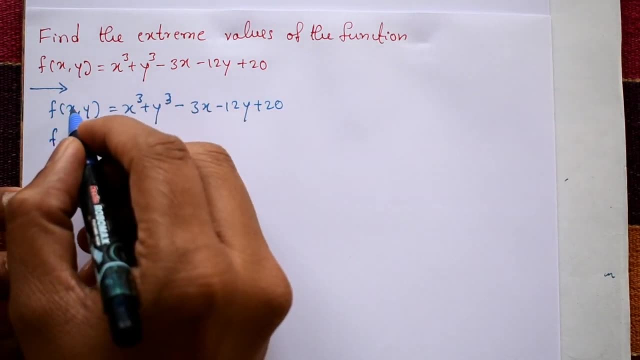 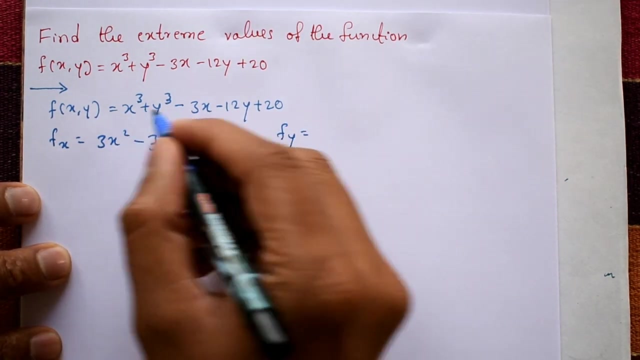 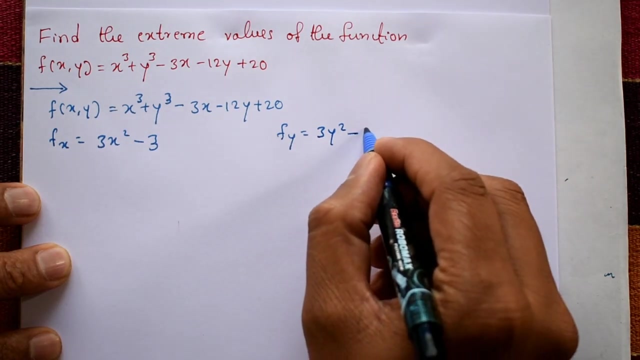 x is treated as a constant 0 minus 3 and y is 0 and this is also 0.. Again, take again this function. Differentiate this function with respect to y. partially. We get fy Do f by do y equal to Now. x is 0.. x is treated as a constant 3y square minus 12 remaining. 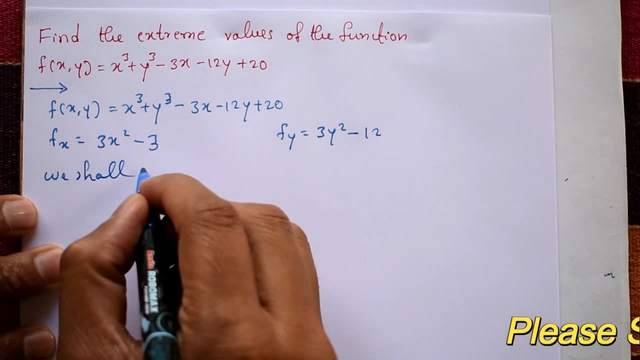 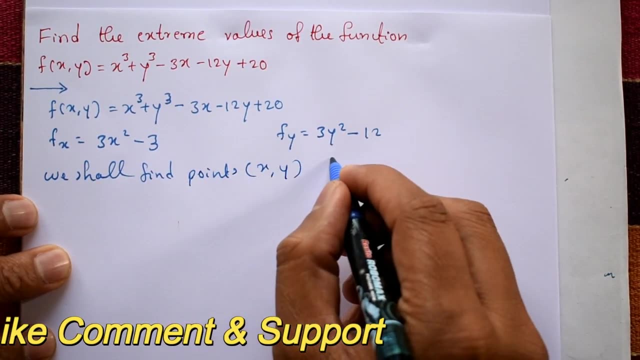 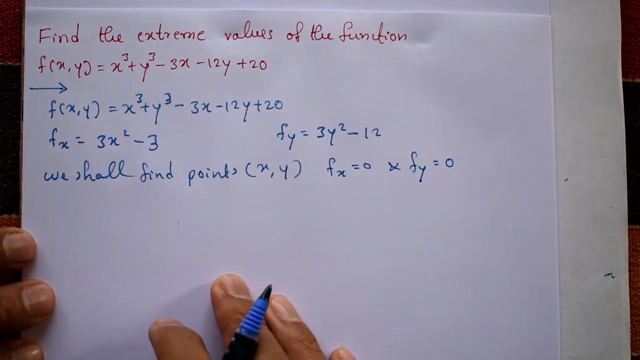 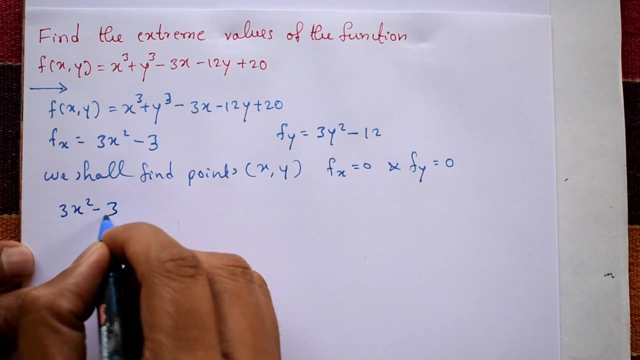 And next we shall find stationary points. Okay, x and y, x and y, That means f of x. do f by do x is equal to 0, and do f by do y, equal to 0.. Okay now, first we take: do f by do y, That is 3x square minus 3 is equal to do f by do x, That is 0 equal to 0.. And second one is: 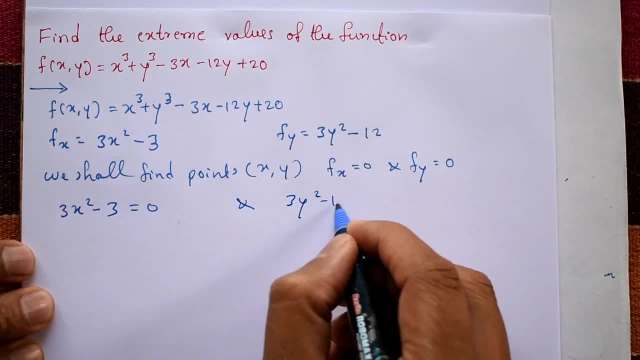 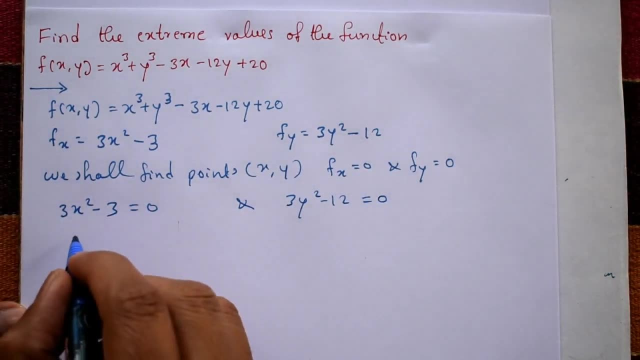 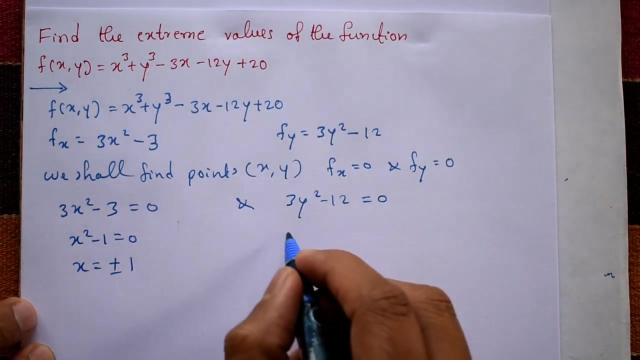 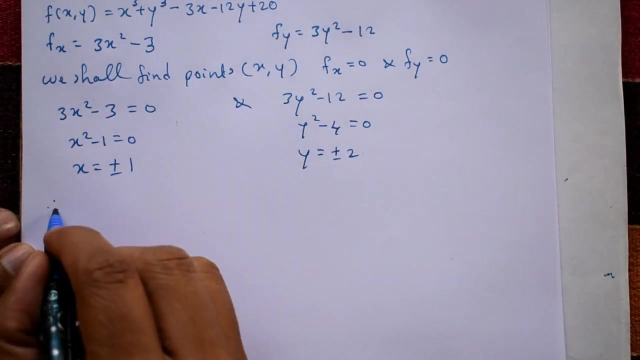 find 3y square minus 12 equal to do f by do y. Do f by do y is 0. That is equal to 0.. Okay, now 3 is common. Take that is x square minus 1 equal to 0, or x is equal to plus or minus 1.. Very simple, This problem is very simple. Now, 3 is take common, That will get a square, What's that? y square minus 4 equal to 0 or y is equal to. again, it is a plus or minus 2.. Now we have stationary points. are 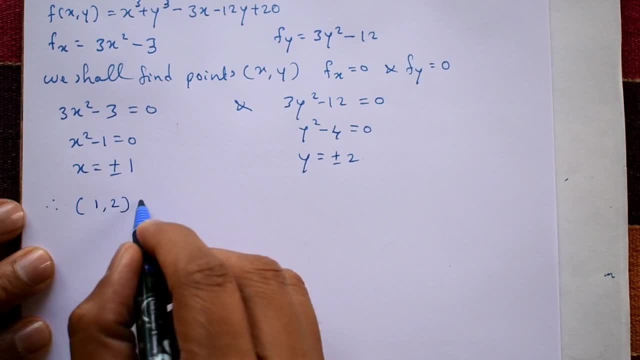 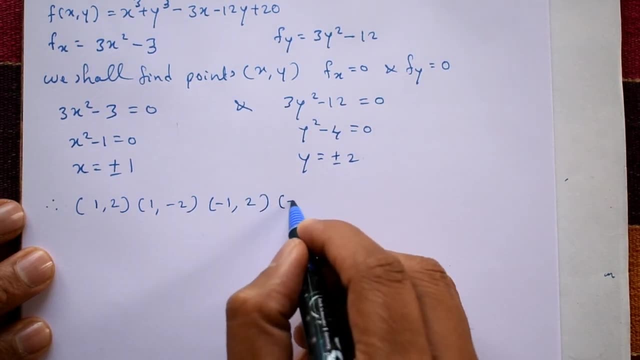 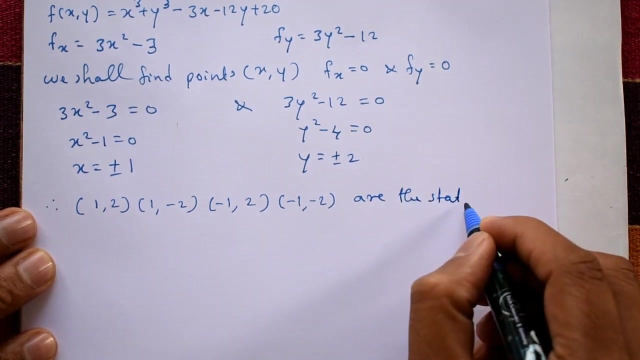 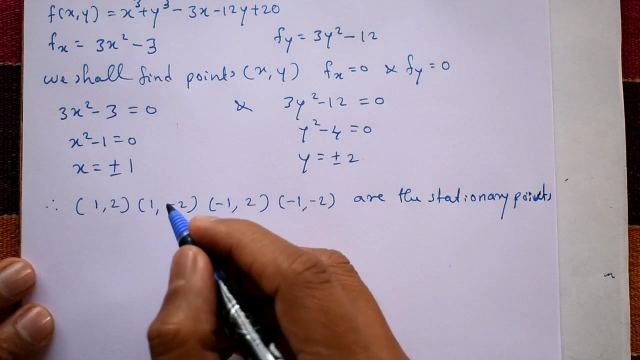 1 plus 2.. 1 and minus 2 and take minus 1.. Minus 1 plus 2, minus 1 minus 2 are the stationary points. Okay, these are a stationary points, Stationary points. Okay, next we need: let I'll take: 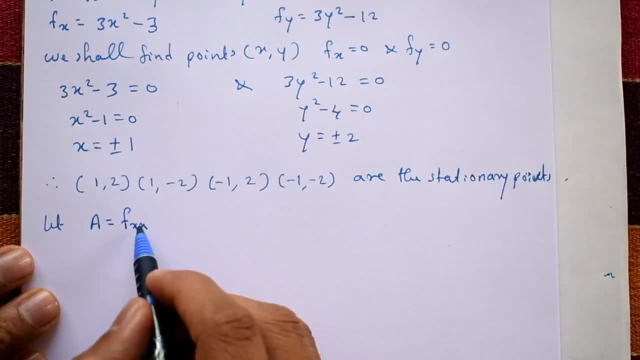 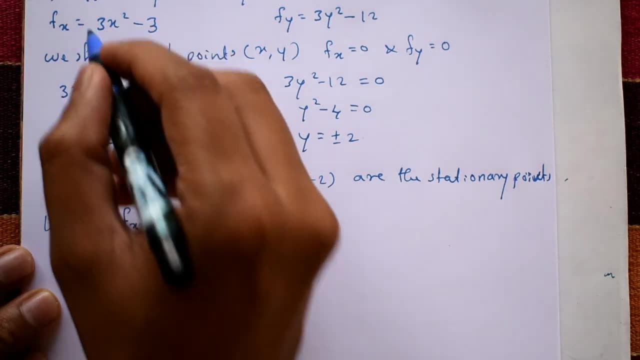 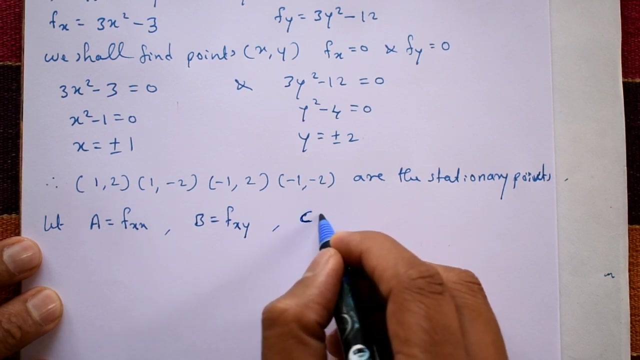 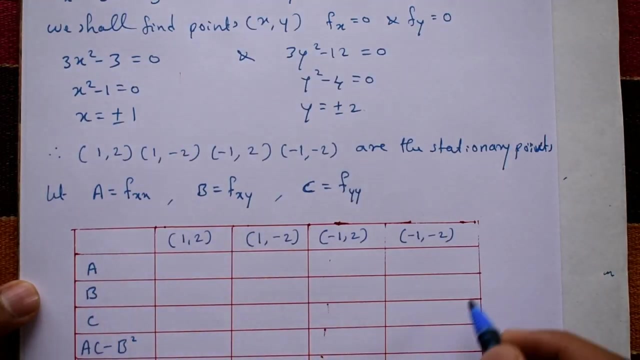 A is equal to this function: differentiate with respect to two times. with respect to x, two times. That is a. Okay. next b is a differentiate function: one time with respect to x, second time with respect to y. Third c, capital c means differentiate function with respect to y partially two times. That is c. Now. this is a table. Now take a. A means differentiate function with respect to x two times One time. with respect to x two times. That is c. Now. this is a table. Now take a. A means differentiate function with respect to x two times One time. with respect to x two times. That is c. Now. this is a table Now take a. A means differentiate function with respect to x two times One time. with respect to x two times. That is c. Now, this is a table Now. take a. A means differentiate function with respect to x two times One time. with respect to x two times. That is c. Now. this is a table. Now take a A. 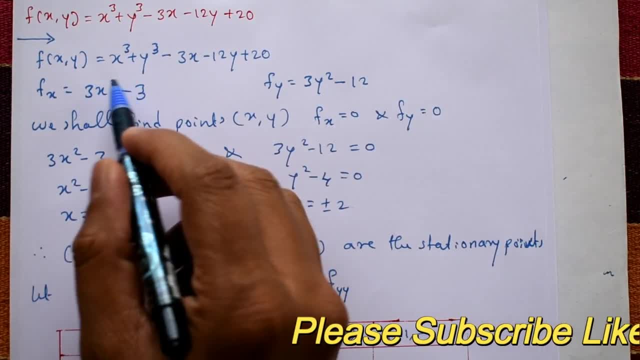 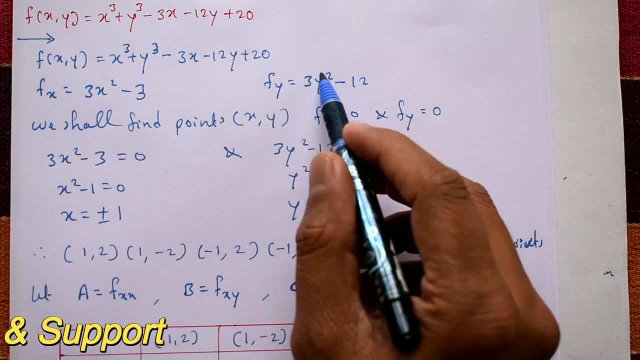 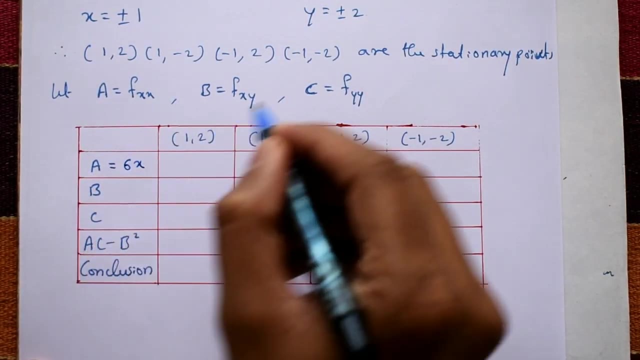 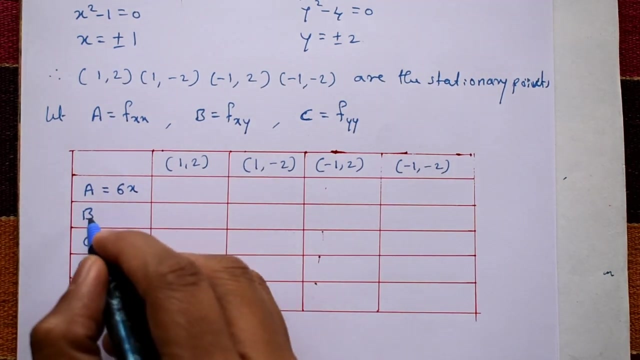 is over. okay, again you differentiate with respect to a, x, we get 6x. or now take this one: differentiate once again with respect to y: partially, we get 6y. now a is equal to 2 times with respect to x. that is a- 6x. now c means this one. with respect to y, again you get c is equal to 6y and b, b means 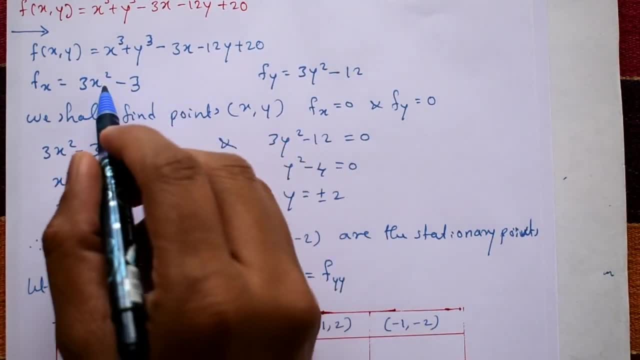 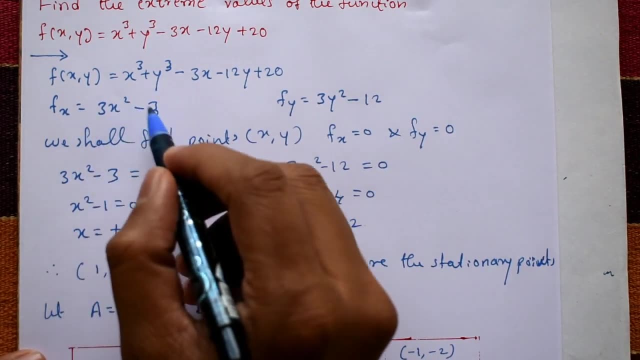 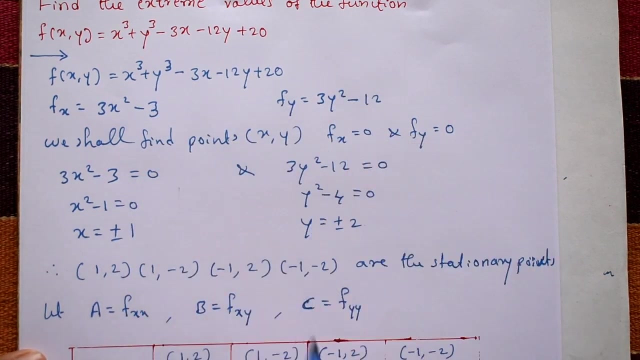 differentiate x and y or y and x. take any one suppose. consider this one: x is over and after. take differentiate with respect to y. now this one is y, already differentiated with respect to y, now take with respect to x. we get the same result. okay, now this is a. b is equal to. 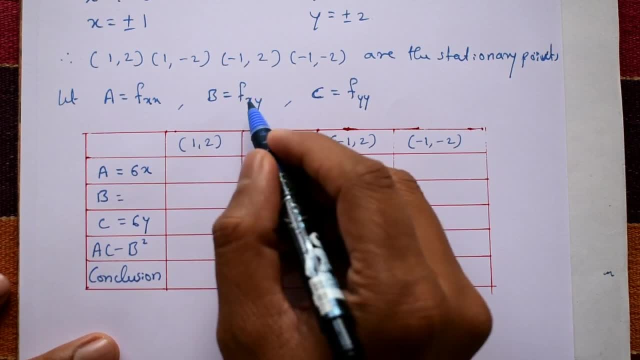 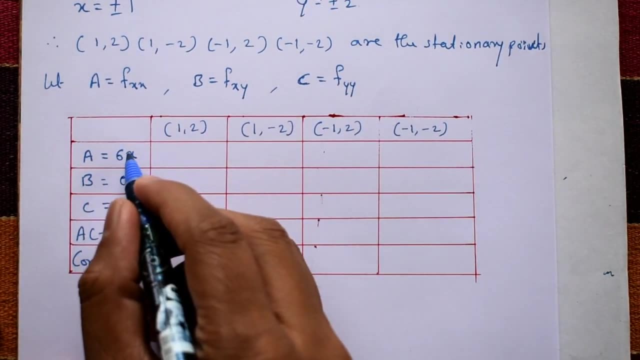 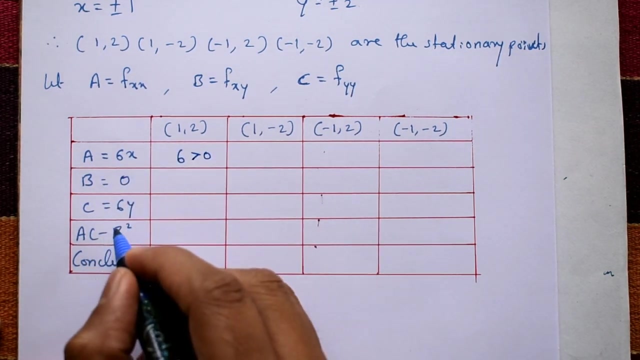 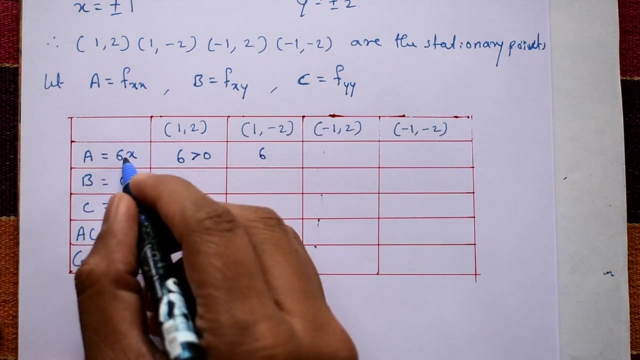 one time x, second time y, or first time y, second time x. that is a 0, okay now. okay now take x and y. substitute: put x is equal to 1, no y variable. we get plus 6. that is positive, greater than 0. now take second one again: put x is equal to 1, 6. take minus 1 means minus 6. 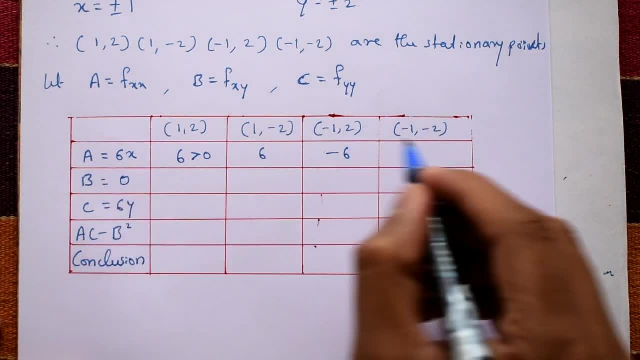 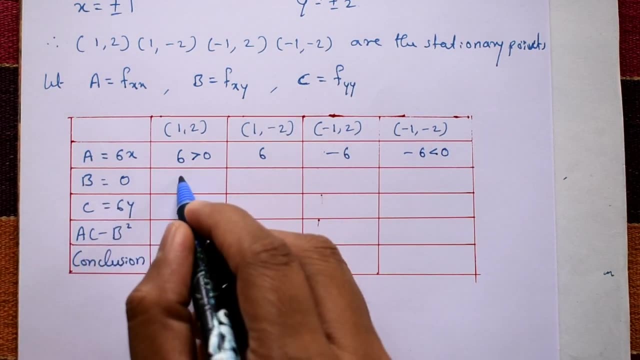 that is less than 0. again take minus 1 x value. that is minus 6. that is also less than 0. okay now take b is a- 0, so all values are 0, no change. now take c: c is equal to 6, y put y values. 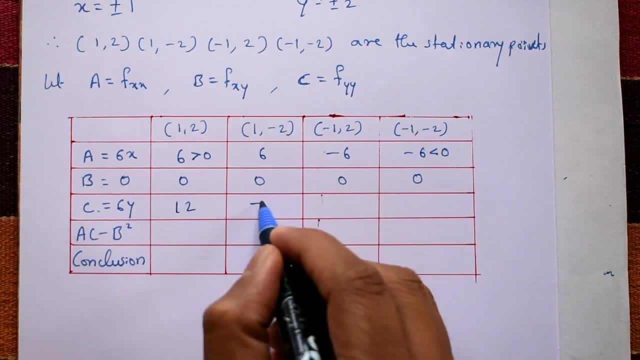 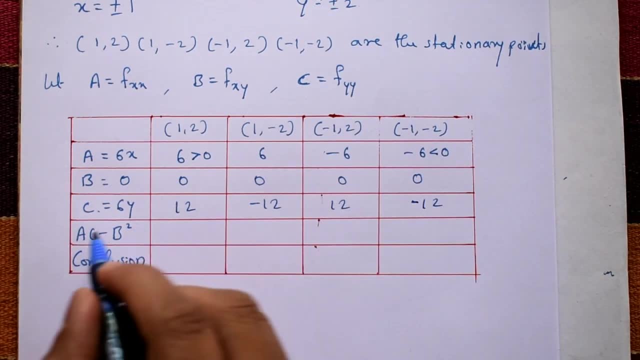 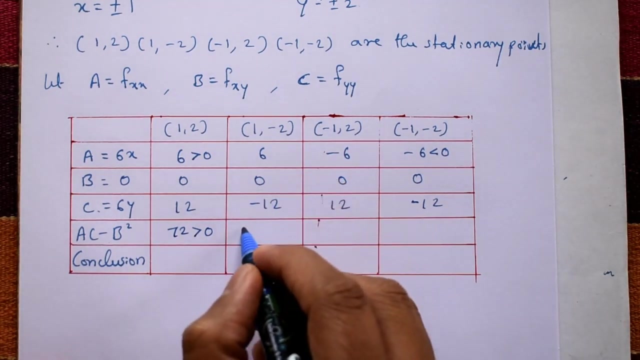 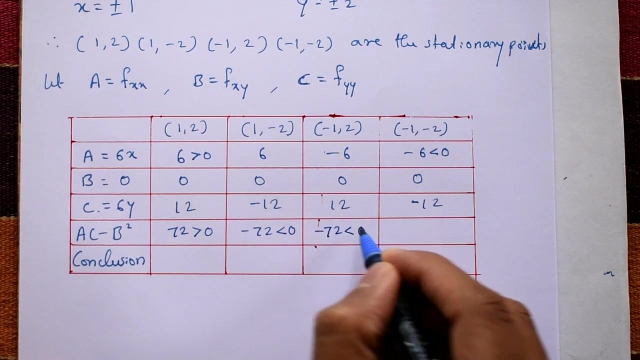 now, this is 12 and this is minus 12. this is plus 12 and minus 12. okay, now ac minus b square a into c: multiplication. and minus b square a into c is a 6 into 12. that is 72. that is positive. again minus 72, that is less than 0. again minus 72, less than 0. 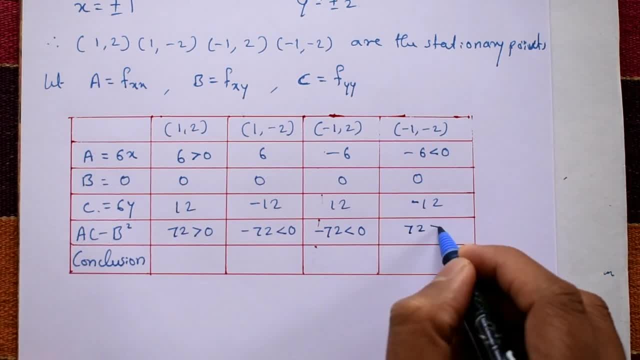 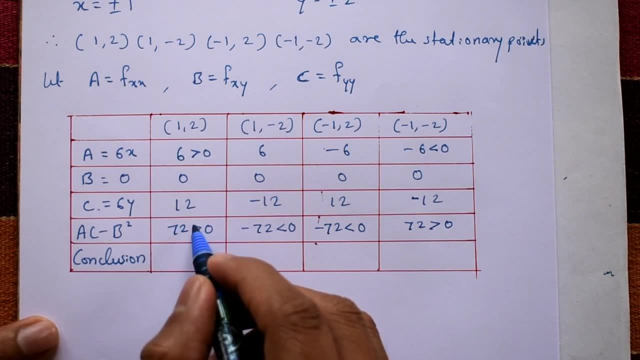 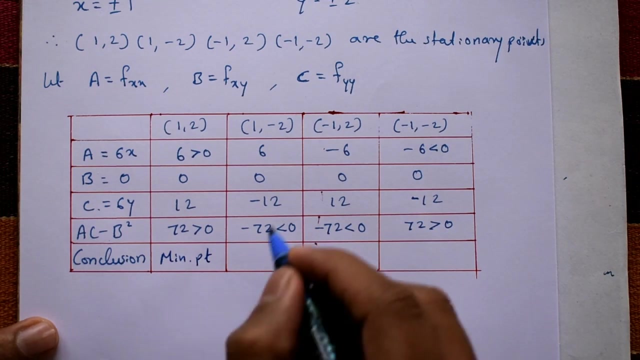 minus 6 into minus 12 is a plus 72. that is greater than 0. okay now, take conclusion: now this value is positive and a is also positive. that is a minimum point, minimum point, okay now. now this value is less than 0. that is a saddle point. 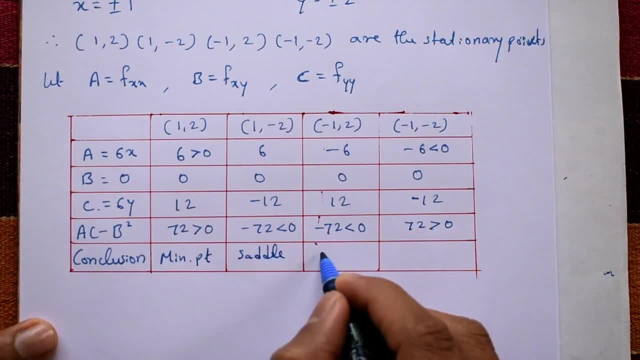 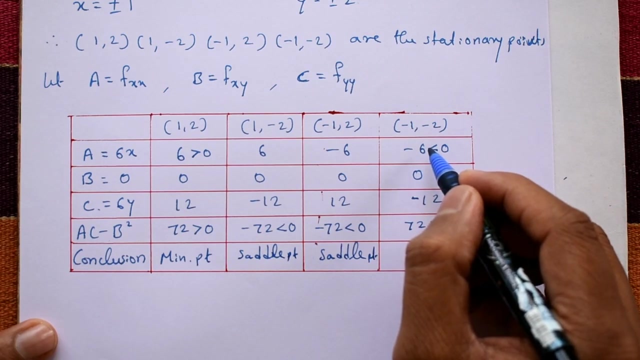 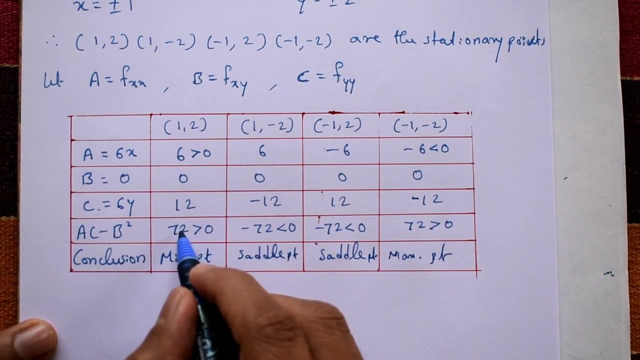 again same: it is less than 0. this value is less than 0, is saddle point. okay, these are a saddle points. now see this: ac minus b square is positive, greater than 0, but a is less than 0. that is a maximum point. now cd these two column: ac minus ac minus b square is a positive and the a is greater than. 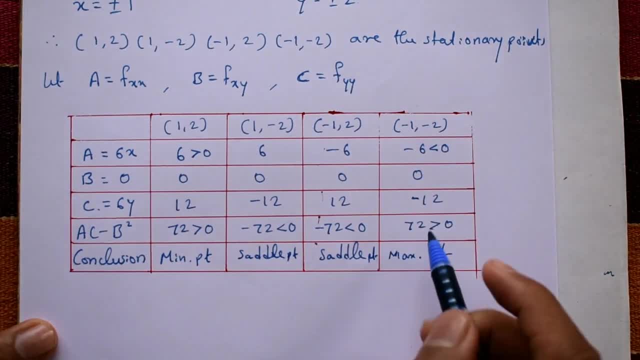 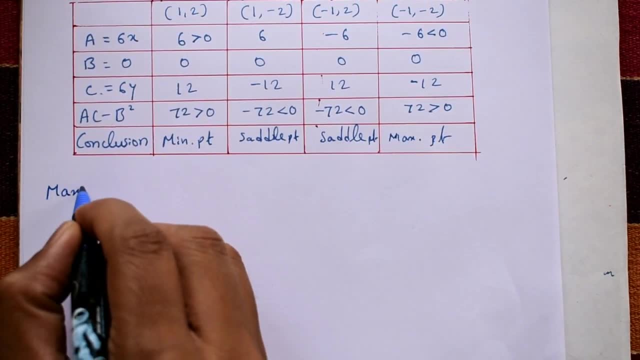 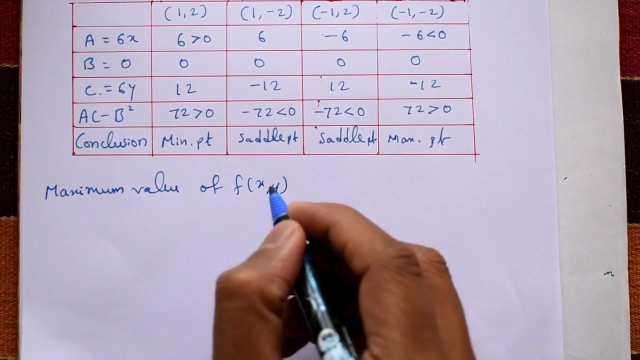 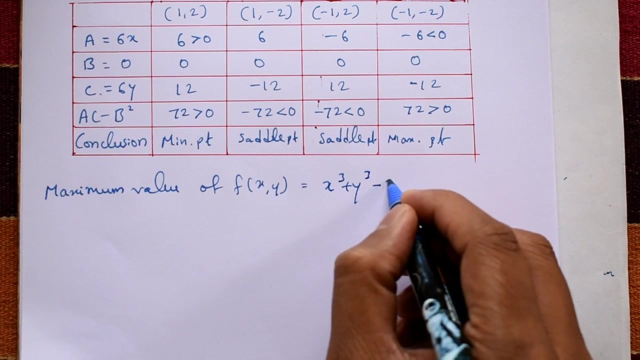 0, that is a minimum. a is less than 0, that is a maximum point. okay, next we require maximum value. minimum value now, maximum value is f of x? y. you know, the f of x? y is a x cube plus y cube minus 3, x minus 12, y plus 20. 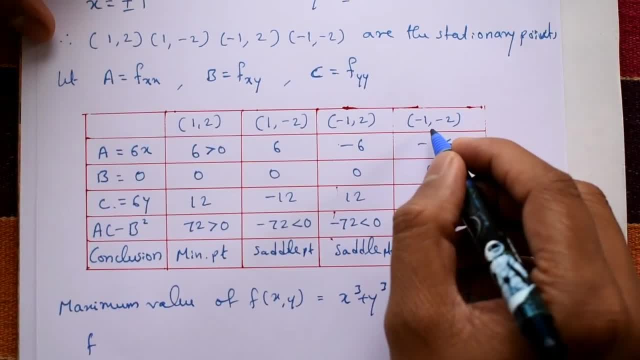 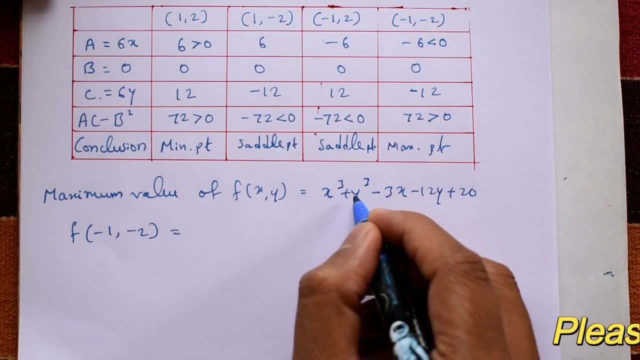 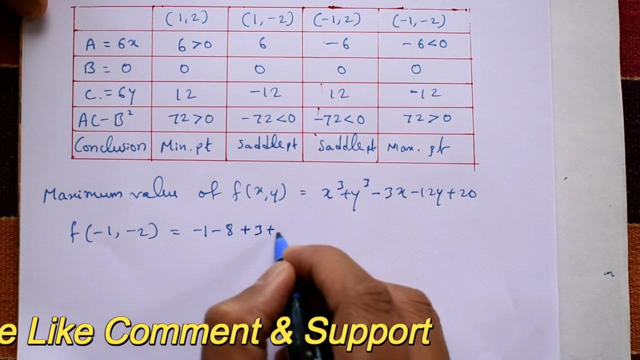 now maximum value. this is maximum points to consider x and y values. x is minus 1, y is minus 2. that is equal to put x and y values. okay, now this is a minus 1 minus 8 and it is a plus 3 plus 24. put x is minus 1, y is minus 2.